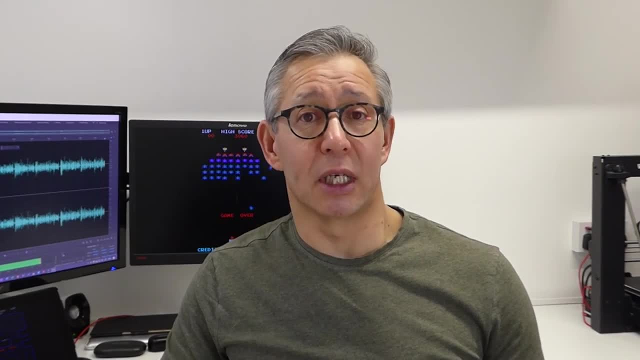 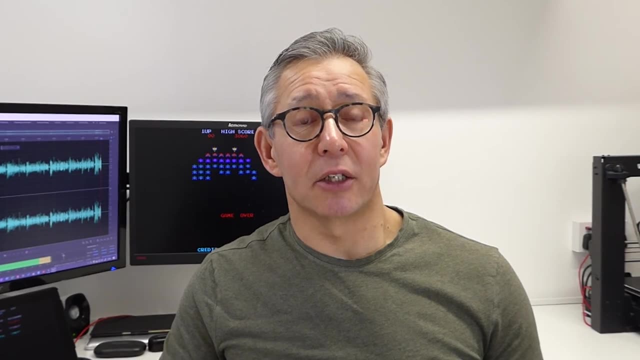 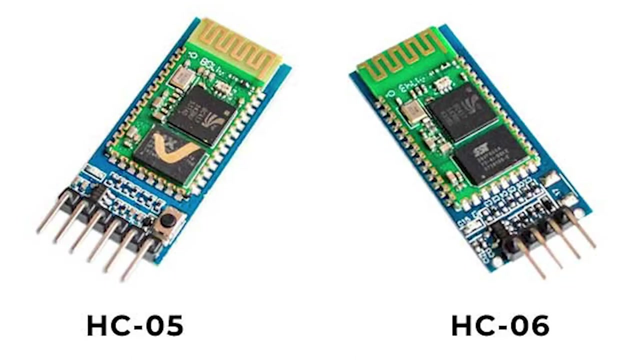 to those And again download all of the code that I've been using and writing for this. So let's get started straight away. Let's connect up our Bluetooth module and get some software running and see how all of that works. The most common Bluetooth modules you'll find 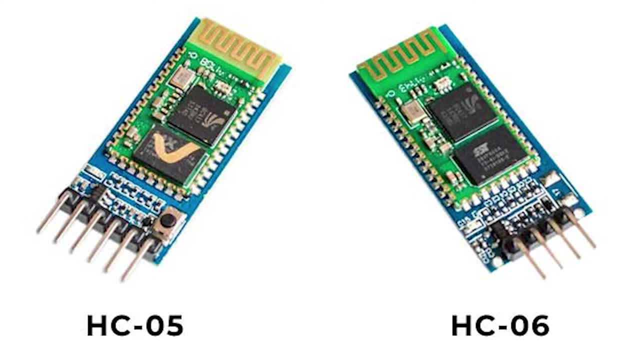 are the 8C05 and 8C06.. And usually you'll buy those on a little breakout board. So on the picture there the actual Bluetooth module is the green circuit board, but that's mounted on one of these blue breakout boards so that we then have some pins that allow us to easily. 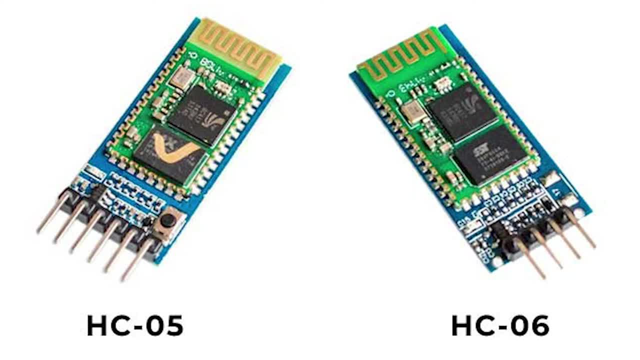 plug it into a breadboard And again, that just gives us the pins that we need to actually drive this thing. Now, if you look, you'll notice that the two devices are slightly different, But as far as we're concerned, in this project we're going to add a Bluetooth connection. 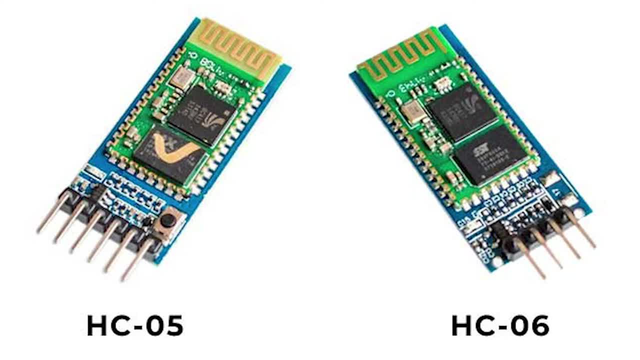 to our Arduino and then we're going to be connecting to it from our mobile device. In that situation, both of those work in identical ways, And that then is in the slave mode, where our mobile phone is going to be the master which is going to initiate the connection. 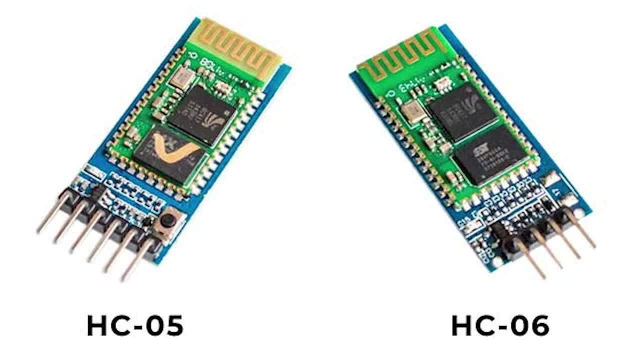 automatically And then be able to then communicate with our Bluetooth module. Now, the 8C06 only works in slave mode, So that's fine for what we're going to do today. The 8C05 has the ability to also work in master mode, So if you did want to connect two Arduino projects together, 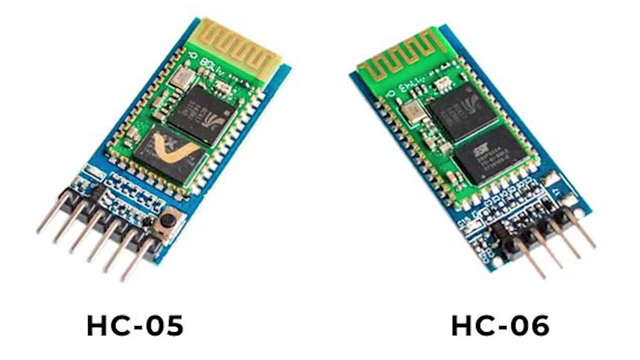 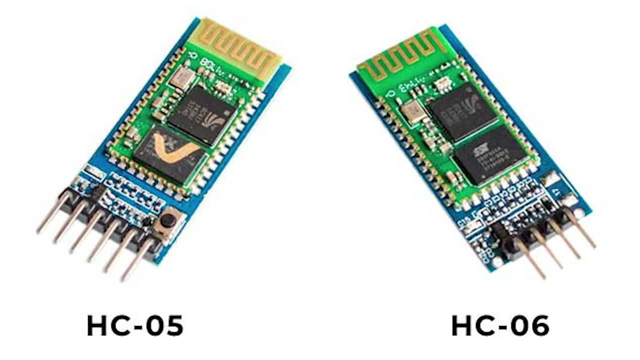 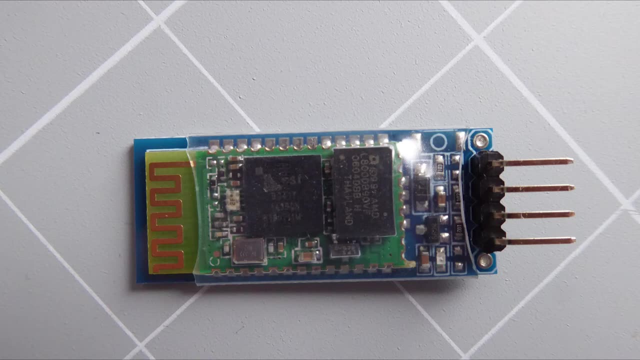 in this course. here, all we're going to do is we're going to be using a mobile app on our phone to connect to our Arduino. So either one of these is absolutely perfect. So I'm going to be using an 8C06 slave only module in this little tutorial, And so I'll, if you're. 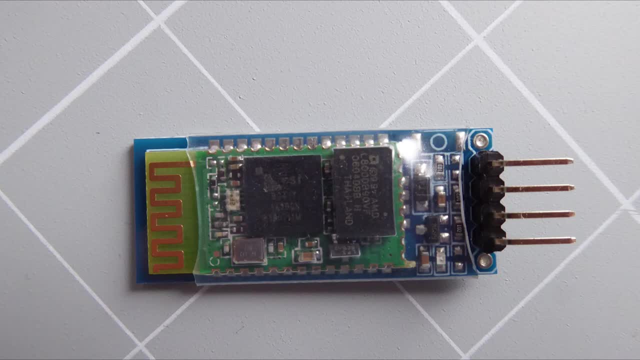 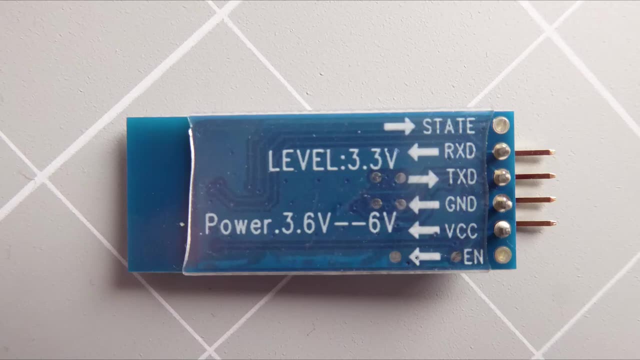 not quite sure which ones to look out for. I'll put some links down to Amazon and eBay in the description below. But if we look at the back end of the module- we've got the back side of the device- You'll see that the actual pinouts are labeled there. So really, 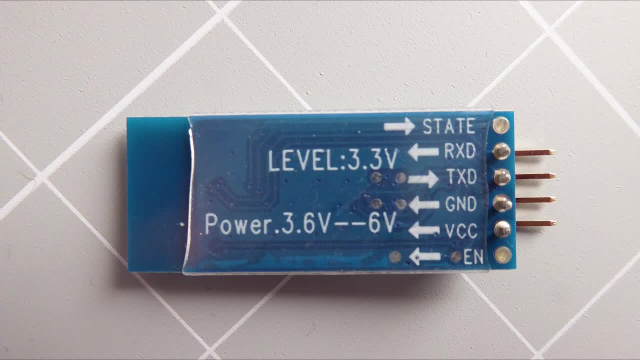 all we need to use are the power supplies. We have our VCC and our ground, and then we have our two data pins, So our transmit data and our receive data, So the TXD and the RXD. The other two pins, which are the enable or key pin and the state output, are not connected. 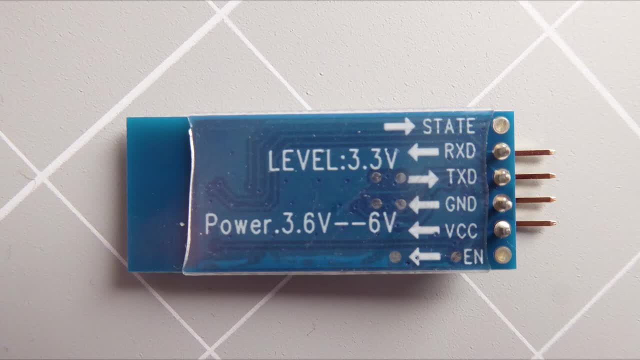 on the 8C06, but they are the two extra pins that you'll find on the 8C06.. So the 8C06, the 8C05.. But, to be honest, at the moment we don't actually need those. So, if you do, 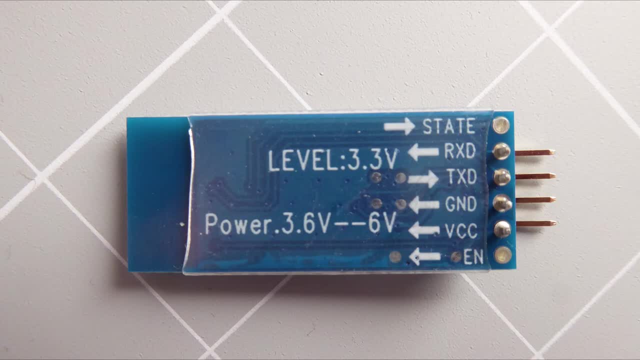 have an 8C05, you can just leave those totally unconnected and the project will work exactly as you'll see in the video. Now, one thing we need to be careful with are the voltage levels. If you look here, our supply voltage can be anywhere between 3.6 volts and 6 volts. 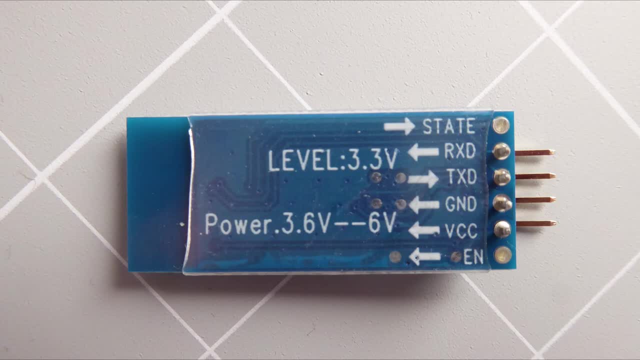 So, again, if we're going to be using a 5 volt system from our Arduino- that's going to be absolutely okay- Our data pins- then if you look at those, they are 3.3 volt digital signals. So using our Arduino with 5 volts coming out of that, we are going to have to step that down to. 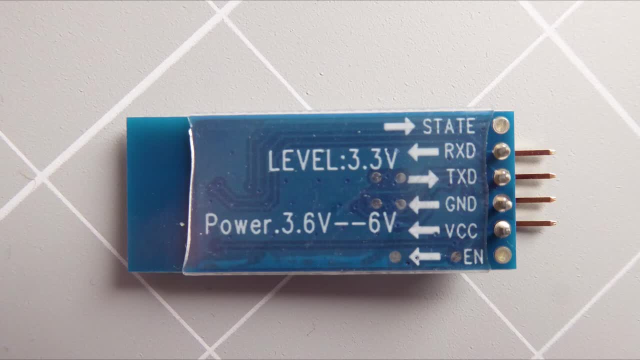 the correct voltage levels, at least on the input into our Bluetooth module And of course that's going to be on the receive data pin, The transmit data pin coming from our Bluetooth module to our Arduino, And we can just connect that directly because that will just be able. 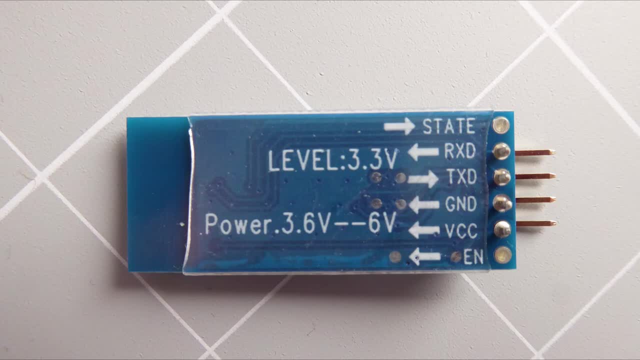 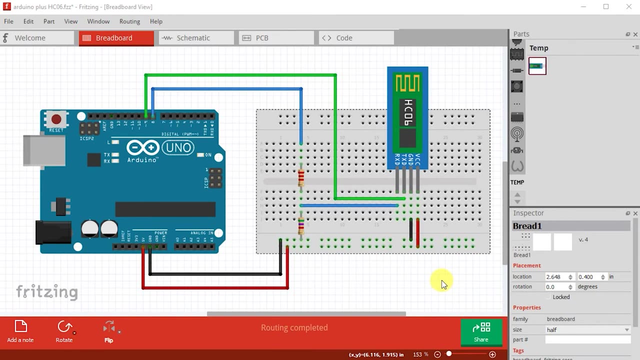 to drive at 3.3 volts, but our Arduino will be able to detect that quite well. So if we have a look at the circuit- and I've laid this out in Fritzing, which is a very handy tool for sort of testing out your breadboards and laying out your electronic circuits- and 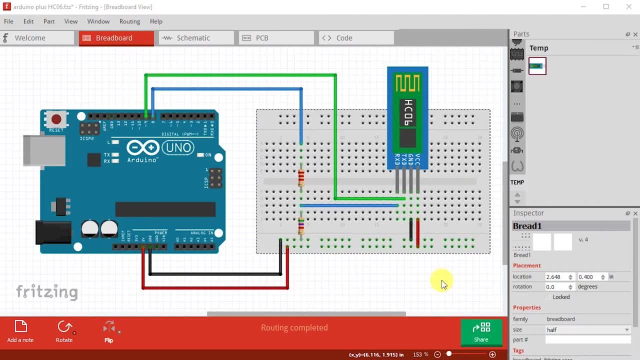 so on. But you'll see that it's a very simple circuit. So our Bluetooth module down here, to begin with, we first of all have to supply it with some power obviously. So we're taking the five volts and ground from our Arduino and we're basically feeding those onto the 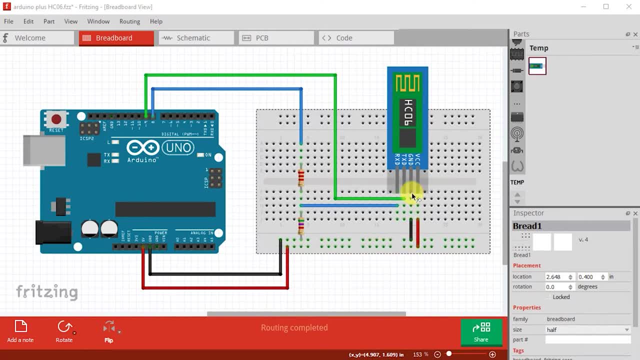 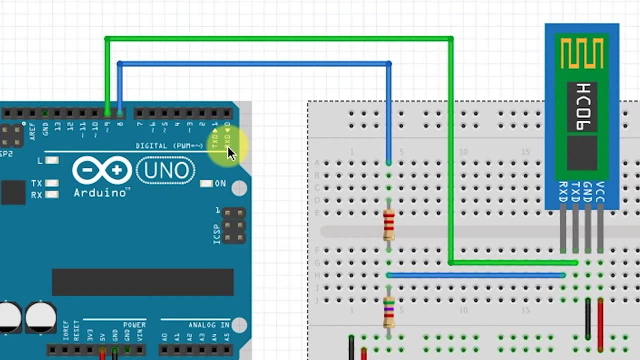 power rails on our breadboard and then into our VCC and ground Now our data. then We could use the serial port. So the Arduino has a hardware serial port built into these two pins. so pin zero and pin one down here. But on the Arduino Uno that serial port is. 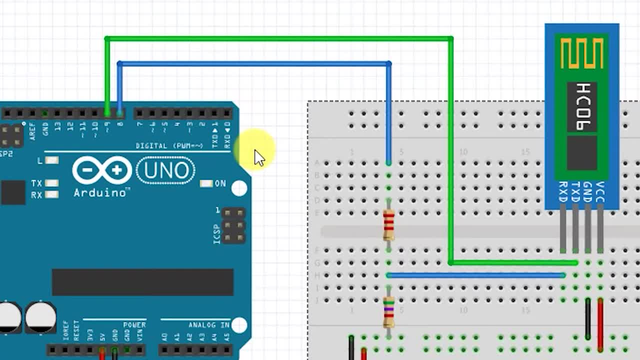 also the serial port on the Arduino Uno. So we actually have the serial port built into the Arduino Uno. so that's basically the serial port built into the Arduino Uno. So we have port used to communicate with your computer. So if we do connect to this serial port, 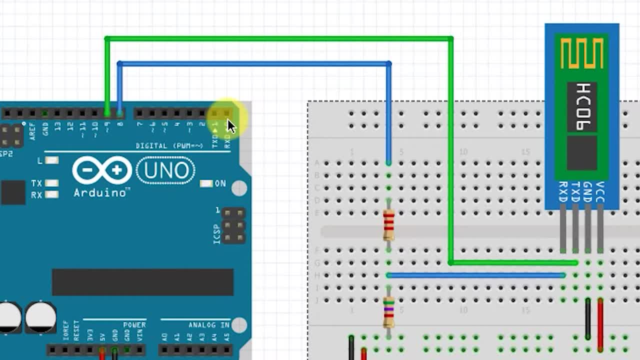 which you can do, and that's not a problem. but if you do do that, then you have to unplug things before you can then communicate with your computer. So, as we want to update the software and so on, we would have to make sure that our Bluetooth module. 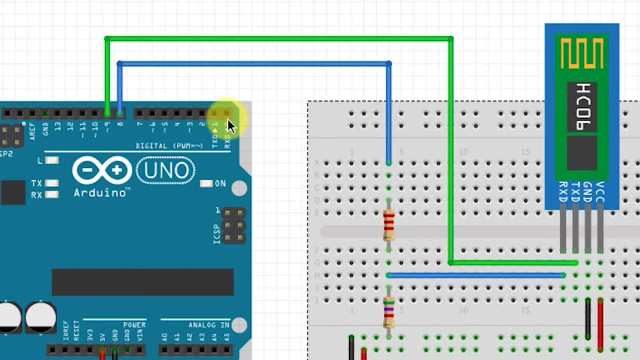 is powered down or disconnected, then upload our software and then reconnect everything up to test it. It would also mean, of course, then, that we wouldn't be able to use the serial monitor on our computer to find out what's happening. So, instead of using the hardware serial port, 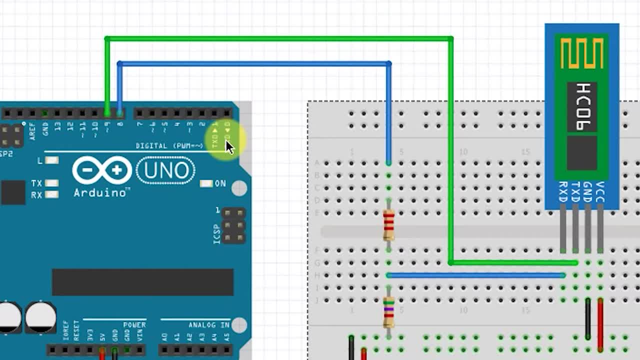 we're going to use a software serial port and that's built into the Arduino IDE as a little package which we can use And that lets us then really create a serial port on any two pins that we want to. So we're going to use 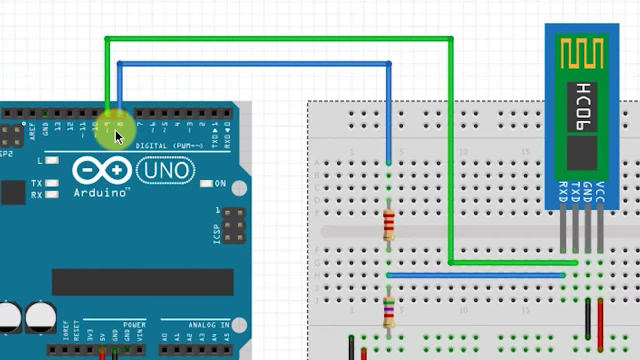 well, I'm going to use pins eight and pin nine and they will then become our serial channel to talk to our Bluetooth module. So I'm going to use pin number eight as the Arduino's transmit pin. So that's going to be information coming out of the Arduino. 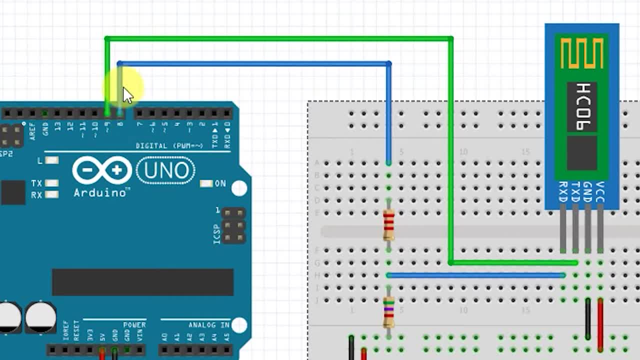 that we want to send over Bluetooth. So this pin here is an output from the Arduino. So remember that our Bluetooth module works at 3.3 volt logic, So we have to send that through a little voltage divider. Which are these two resistors here? 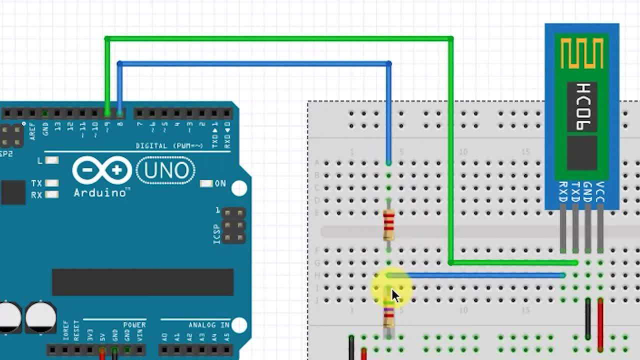 So from our signal coming out through a resistor, through another resistor, down to ground, which means that when we tap off in the center here, if we choose resistance value, so I've got a 2.2K and a 5.7K resistor here. 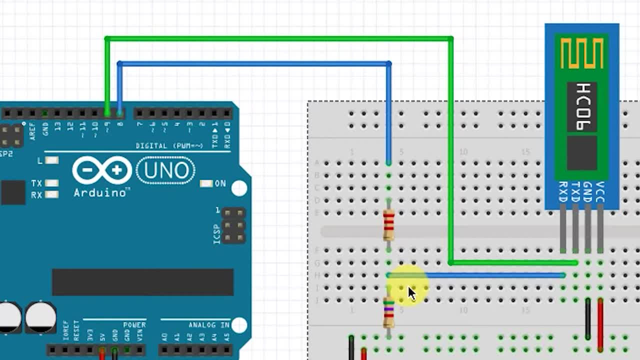 And if we use those as a voltage divider, that should give us around about our 3.3 volts, And again, it doesn't have to be exact as long as it's around about that value. So we're tapping then off from that center point here. 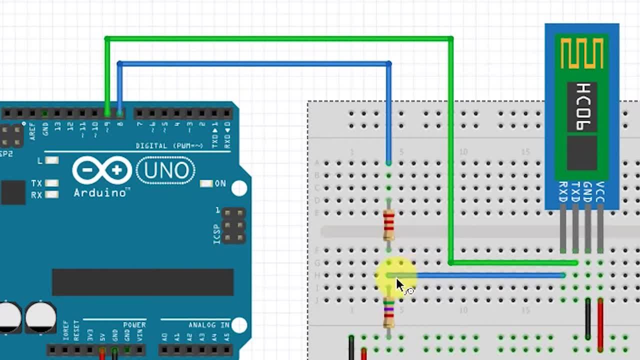 and we're going to tap off from that center point here, and we're going to tap off from that center point here and we're going to tap off from that center point here in our potential divider, which should then, as I say, 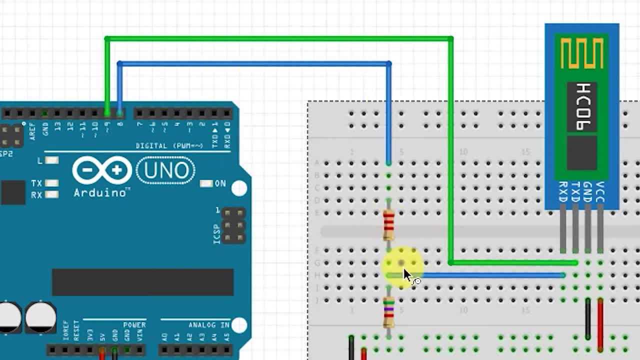 voltage shift our five volt data signal coming out of here to a three volt data signal which we can then feed into the receive data pin on our Bluetooth. So remember it's important here that the transmit pin on our Uno or our Arduino is connected to the receive data pin. 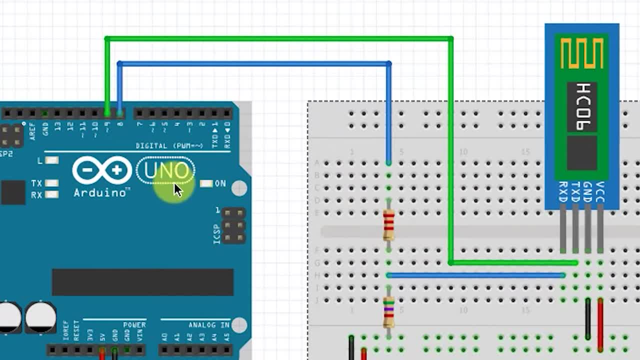 on the Bluetooth module. So, if you think about it, the Uno is transmitting data and the Bluetooth module is receiving that data. So the only other connection in the circuit then is from the transmit pin on the Bluetooth, the HCO6, and that is simply connected directly onto pin number nine. 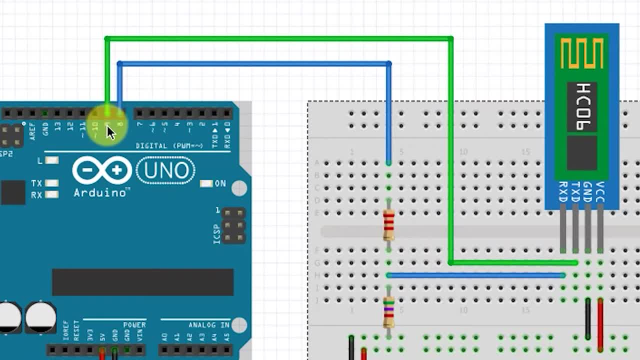 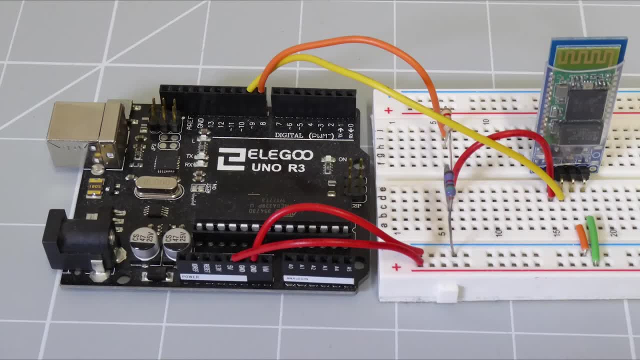 which will be the receive data pin on the Arduino, And that really is the whole circuit that we need. So this is that same circuit built up on actual breadboard with components And, as you can see, there's not very much to that. 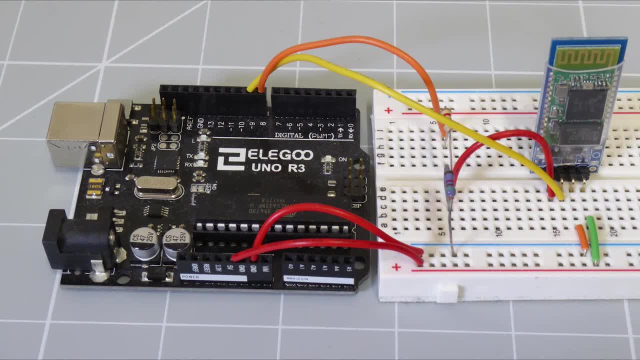 But it does mean, then, that we are ready to start making this work. All we need to do is to add the code to drive it. So let's get straight into that and get some data moving. So this is just a very simple Arduino sketch. 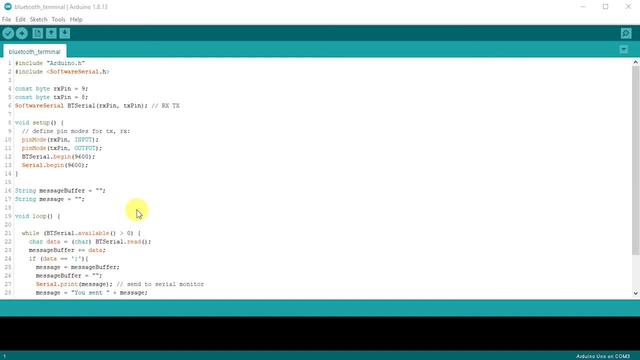 and really what we're gonna do is we're going to connect to our Bluetooth module, We're then going to listen to see if anybody is sending us any data, and then we're gonna going to print that out back up to the PC through the serial port. So let's have 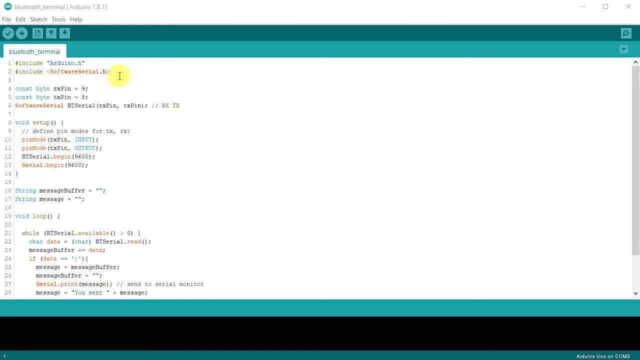 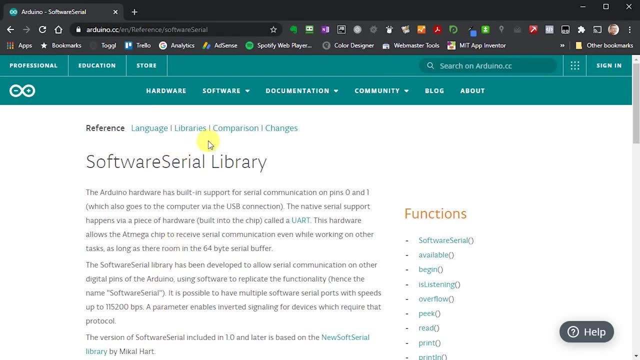 a look at the basic structure then. So we need to use this software serial library. So if I bring that up on on the Arduino website, So this is the software serial library and you can see there that it provides a number of functions which we 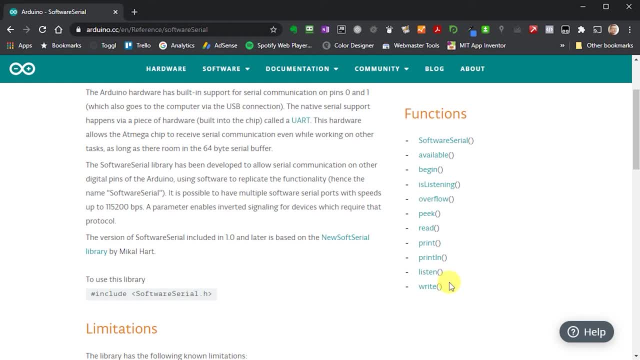 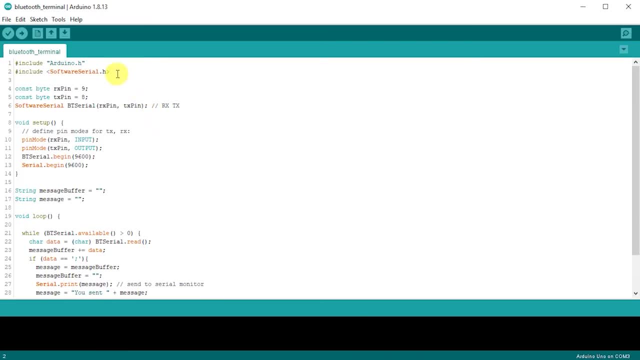 need to use to to communicate over Bluetooth. So let's go back into Arduino and see where that actually happens then. So we import our library here. We then need to tell our software serial module which pins we're using for our receive and transmit. So I'm just defining our two pin numbers here. So we're saying: 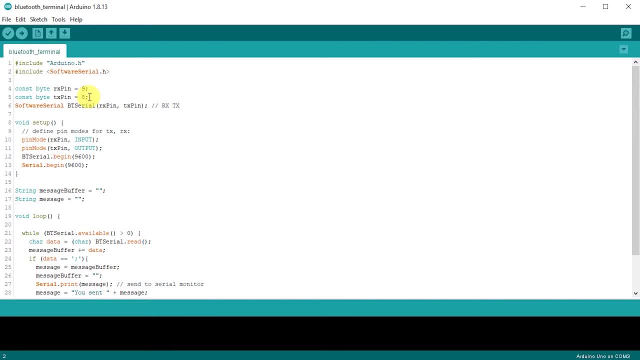 that our receive pin is going to be on pin 9 and our transmit pin on pin 8.. We're then instantiating one of these software serial objects. So we're saying we're creating a variable called bt-serial, So that stands for my Bluetooth serial link, That is. 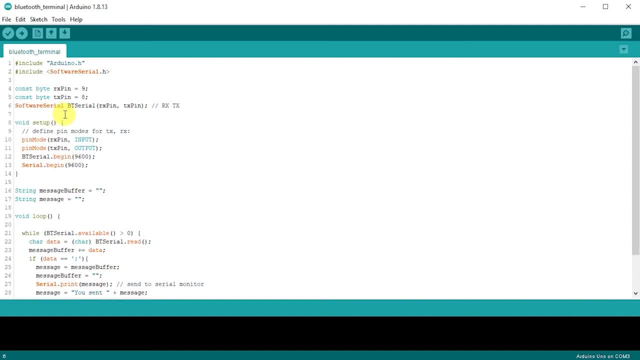 going to be an instance of this software serial object For its constructor, then we need to tell it which pins we're using for our receive pin and our transmit pin. So at that point we now have bt-serial, So this variable here is now an instance of this object. So we're going to be using our two. 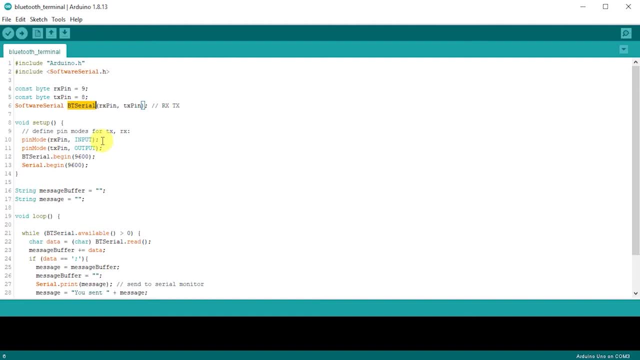 pins. So there are our receive pins, and then the bt-serial pins pin needs to be set up as an input. our transmit pin needs to be set up as an output. Now, by default, the Bluetooth modules talk to the Arduino at 9600 baud. 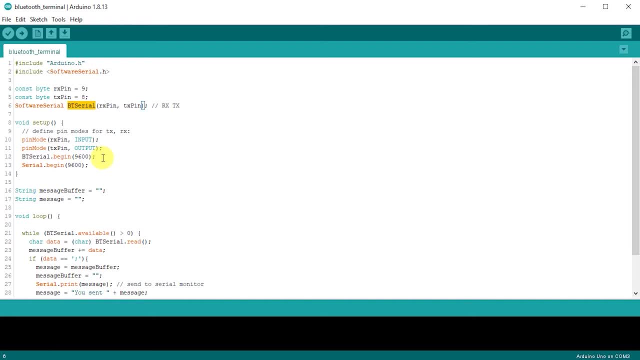 We can change that and, as I said, that, that's one of the things I'll be looking at in another video, where we can actually communicate directly with the Bluetooth module and change its settings. But when you first buy it, it should come along and it should be set up at 9600 baud. So we're saying here, we're going. 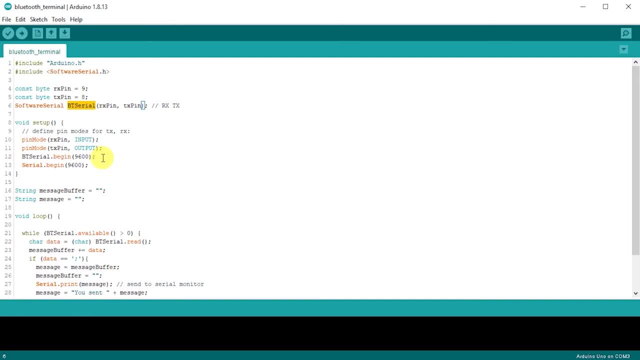 to start our Bluetooth serial object and we're going to begin transmission and we're telling it what baud rate we're going to use. I say I'm also then going to be sending data back up to the PC for the serial monitor. so again, we're going. 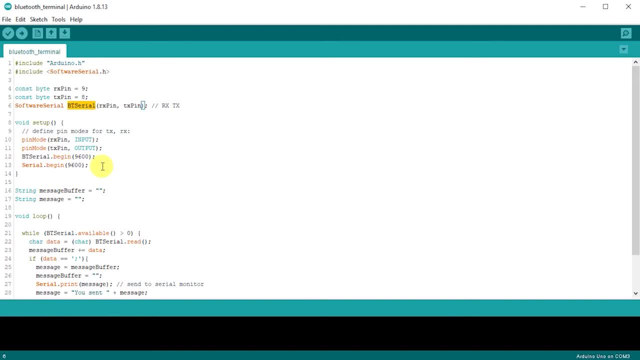 to start off the hardware serial channel, and we're going to set that up at 9600 baud as well, just just to keep everything in the same, And that's that's the end of the video. Thank you very much for watching and I'll see you in the next video. 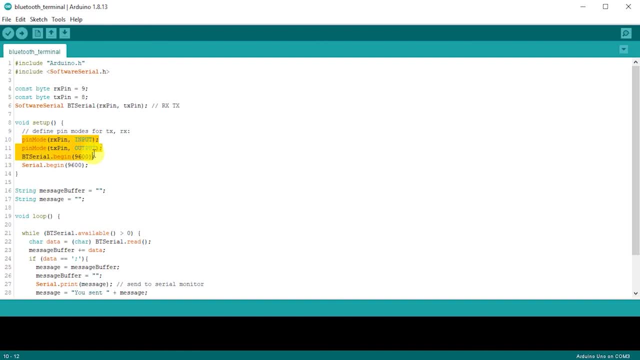 That's basically our setup done. That's all we need to do. So these three lines here, basically, after we've defined our software serial object, that's all we need to do to get it up and running. So the actual loop. then all I'm going to do 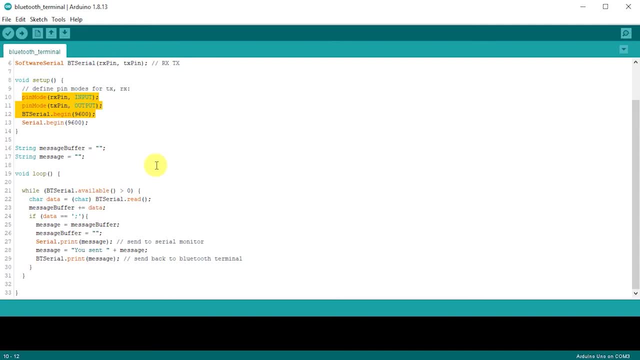 here is: I'm going to sit receiving data until I get an end of message character. So what's happening? So we're using these two global variables here to build up the message. then inside our main Arduino loop we're a little while loop here. so we're saying: so we're using this from this method of our software serial. 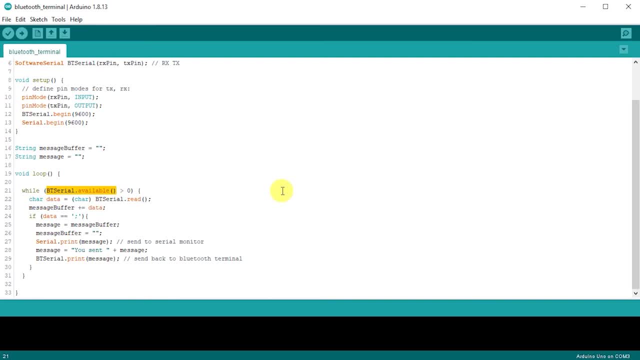 object and that basically tells us if we call the available method that will tell us how many characters are waiting for us to read. So all of this happens asynchronously to our Arduino code, so as the Bluetooth module receives data and it transmits it across to the Arduino. but this blue, this software serial class. 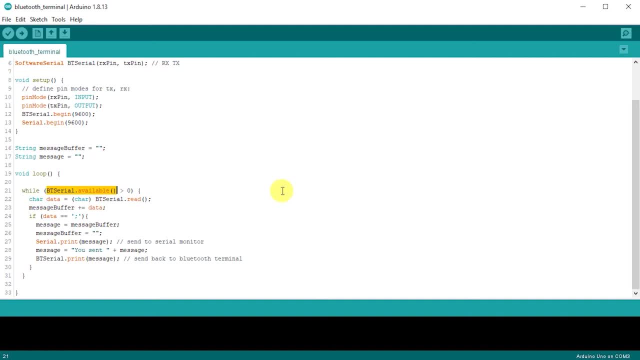 or the object simply sits there collecting that data and making it available then for us to read. So that says that. so if we get that value coming back greater than zero, that means that there are characters in the serial buffer waiting for us to deal with them. So all we're saying then. so while we 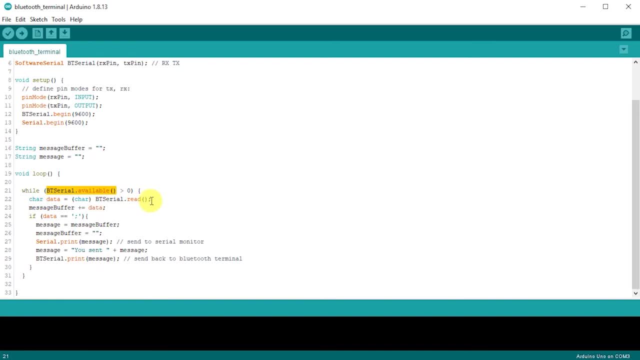 have some more data to read. we're going to read the next data, that we're going to read The next character. so I'm saying here I'm creating a variable data and that's going to be equal to the next character in the serial buffer and then adding: 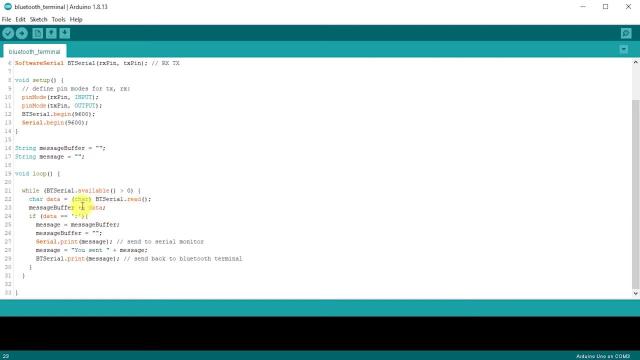 that on to my message buffer, so I'm as well buffering it here in inside this variable, and then I'm using a semicolon as my end of message character. so we're basically gonna sit in here. if we've got characters available, we read it in and 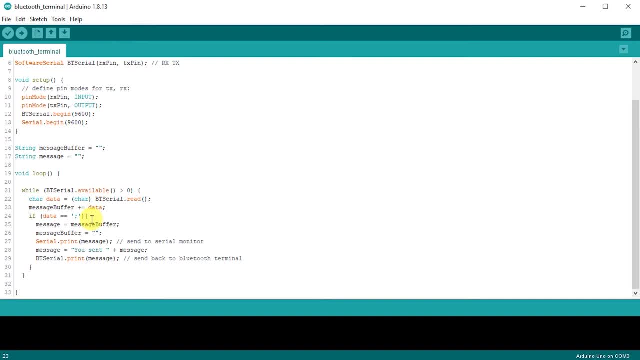 we add it on to our message. If we just received a semicolon character, then we're going to do something down here. otherwise we simply just keep looping round reading the characters until we eventually do get a semicolon character. At that point this test becomes true. so we come in here. we store the current buffered message. 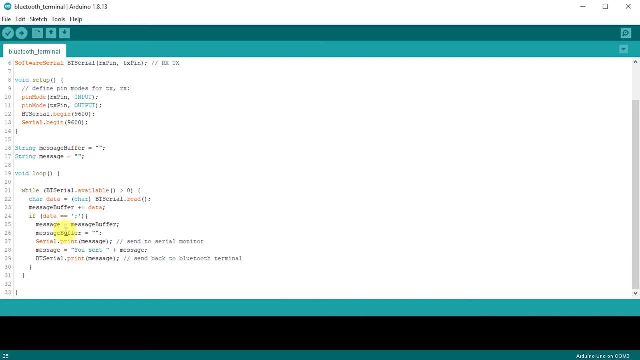 inside this variable message and then we clear our message buffer variable. so it's right then ready to start buffering up the next message. We send the message then up to our serial monitor so we can see that on our PC. This is a message coming from our Bluetooth connection to the Arduino. 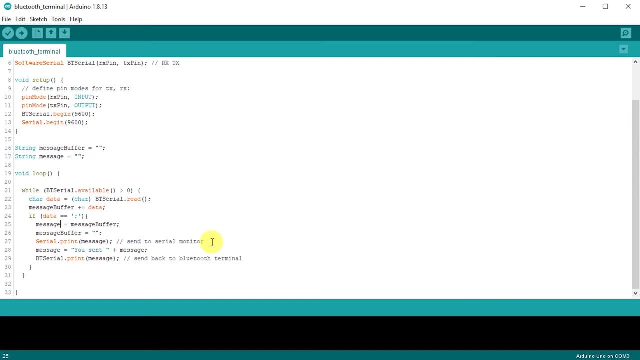 so that will then tell us what has been sent to the Arduino. We're going to send a message back up to the Bluetooth terminal. really, we're gonna have a little Bluetooth terminal running on our phone that's going to allow us to send a message down to the Arduino and then on our PC. 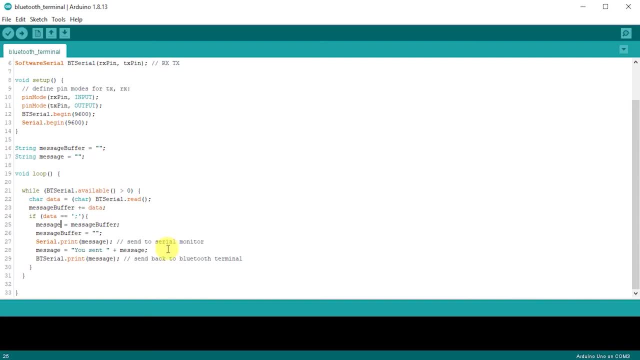 Once it receives that message, it's going to send a message back up to our phone and we'll be able to see that appearing then on the screen on our phone. And again then we're using the print method of our software serial object and that allows us to send a text message back up over our Bluetooth. 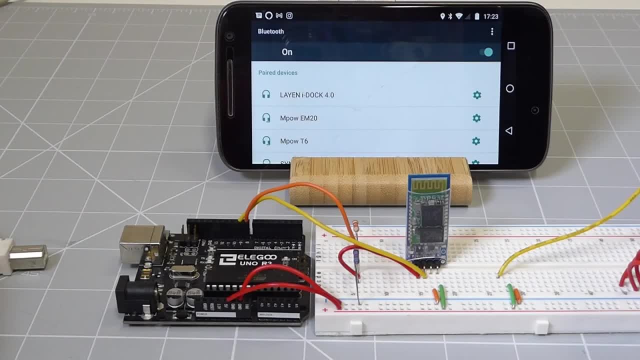 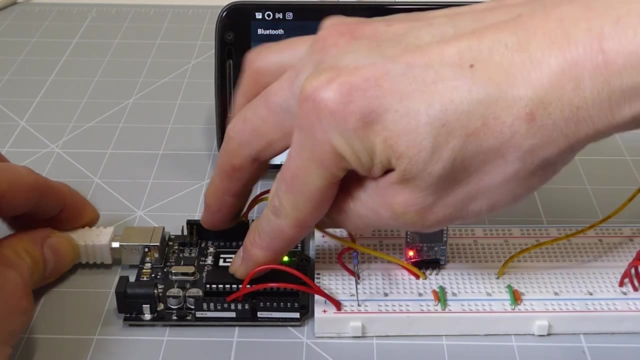 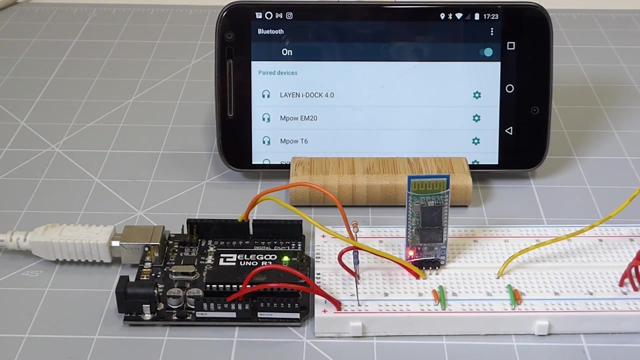 So, coming over to the actual circuit, the very first thing we need to do is to pair the two devices, So this enables the phone to actually talk to the Bluetooth module. So if I power on the Arduino, you'll see that we get a flashing red light on our module and that means that it is now in pairing mode. 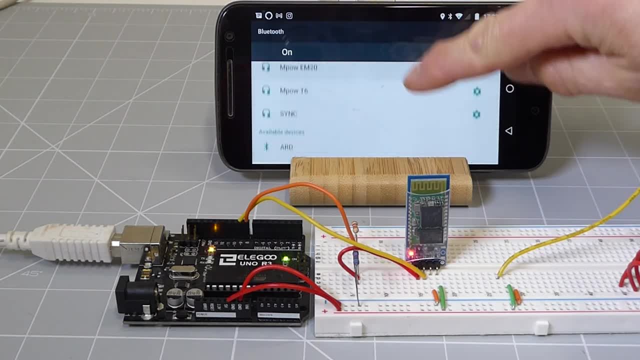 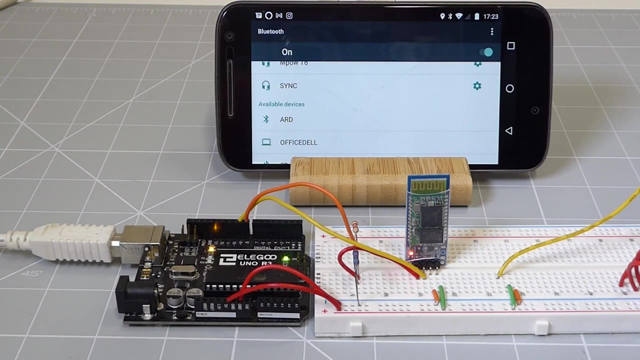 So if I come on to my phone and into my Bluetooth settings, we should see in available devices, we should see something that will relate to your module. Now I have already set up my module and again I'll talk you through how to do that and how to set its device name in a different video. 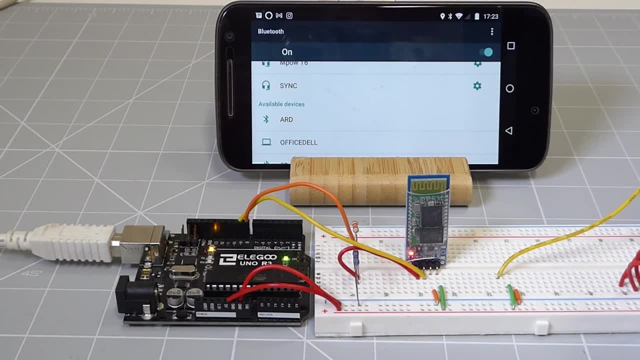 And mine is coming up as this ARD for Arduino. Now you will have something coming up there which will be fairly obvious that it is your Bluetooth module. If not, obviously just have your screen with its available devices. then power up your module and you should see a new device. 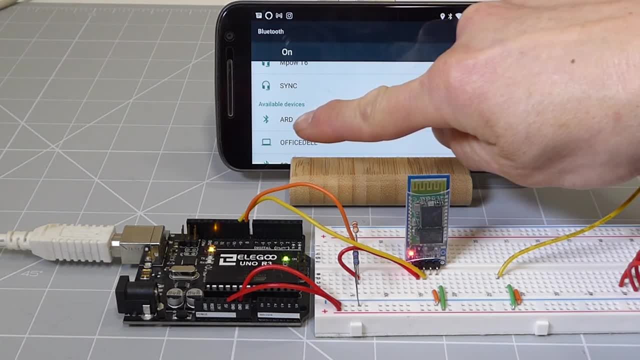 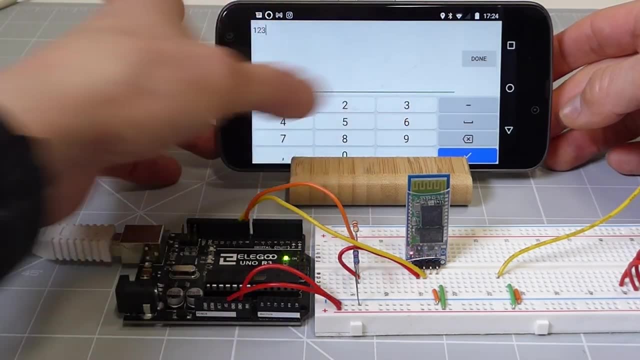 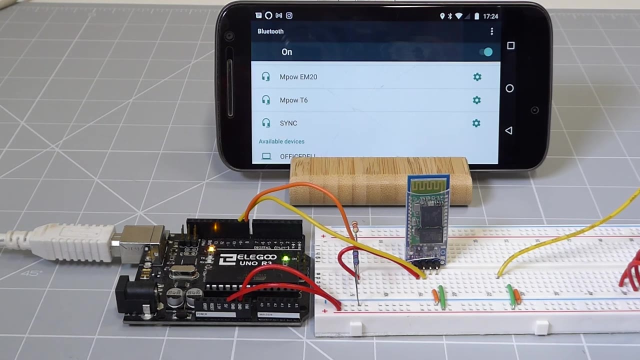 popping up in the available ones and all we need to do is we need to select that and then pair with it, and the pairing code is usually one, two, three, four, and if we okay that and then okay that, we should then find that we are now paired. 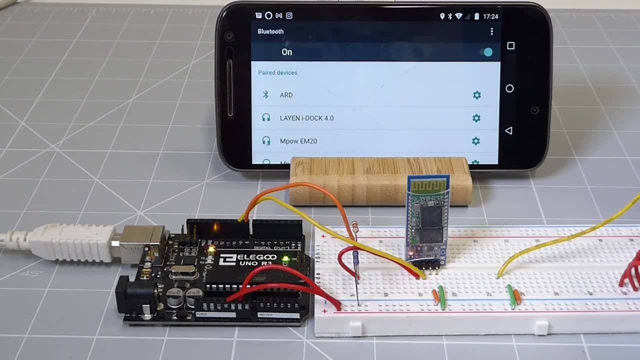 with our with the module. okay, so it's not coming up in my pair devices. we haven't yet created an actual connection to it, but we have paired our phone with it, so it is not able to make that connection. so let's have a look and see. 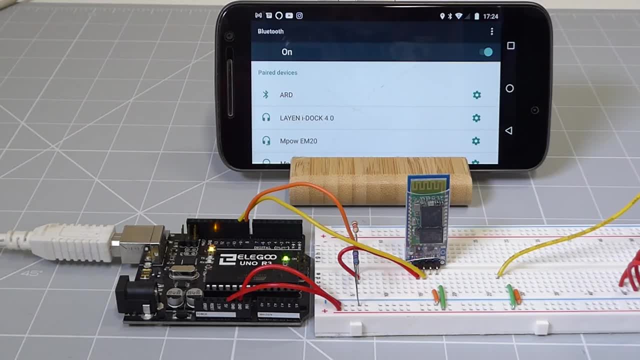 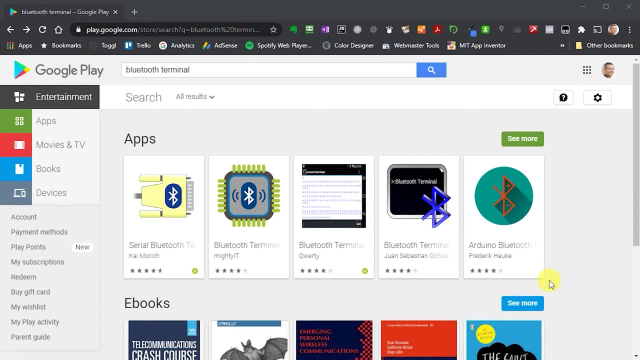 how we actually connect and start sending some data. so to actually communicate with our Arduino, we need a little bit of software running on our phone. so I'm going to just simply start with this idea of a Bluetooth terminal. so if you go to whatever app store you use for your 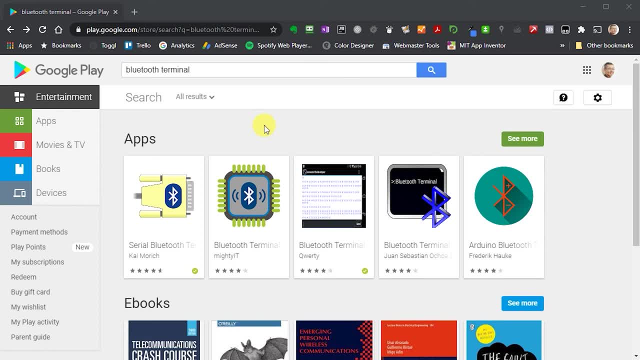 phone and search for Bluetooth terminal or serial Bluetooth terminal, you should get a range of apps turning up, and the one I'm just going to use is this first one here, the serial Bluetooth terminal by Kai Morich. no particular reason I'm using that, it's just that it does have the features I need. so if I go into it, 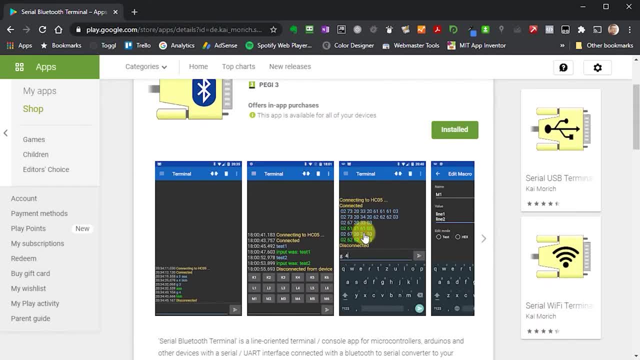 the features we want, then it needs to be a terminal where we can type in messages and then send them to our device and, of course, be able to see the messages connected to RAM protection and then we can then have a look at that with the coming back from our device And the important feature that we do need to do. if I expand this, 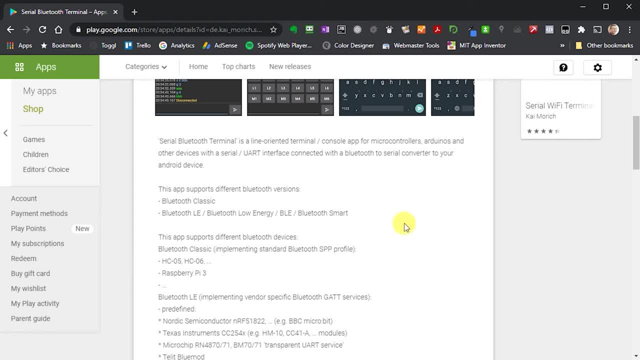 read more bit here. there's a number of different versions of Bluetooth, So we have our original sort of Bluetooth and then our Bluetooth low energy versions, which are slightly different. So you do need to make sure that the app you use is compatible with Bluetooth Classic. 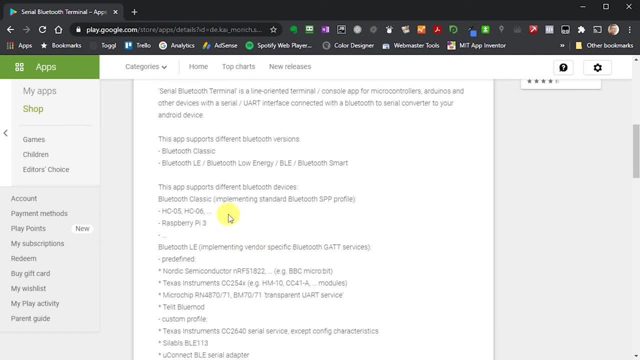 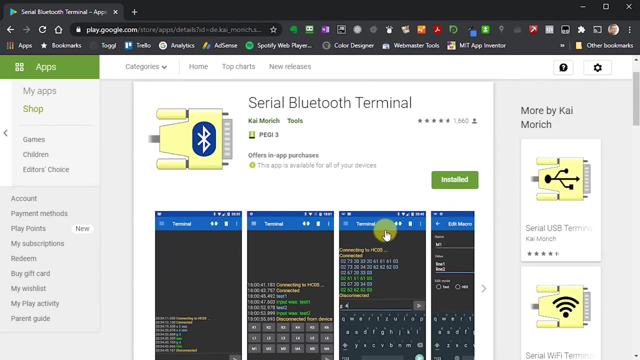 Now you can see in here, then this one does support that, And it does specifically mention that it is able to talk to the HCO5 and HCO6 Bluetooth modules. So this one's going to be fine for us to use. So once you find one that is suitable, then just simply install that onto. 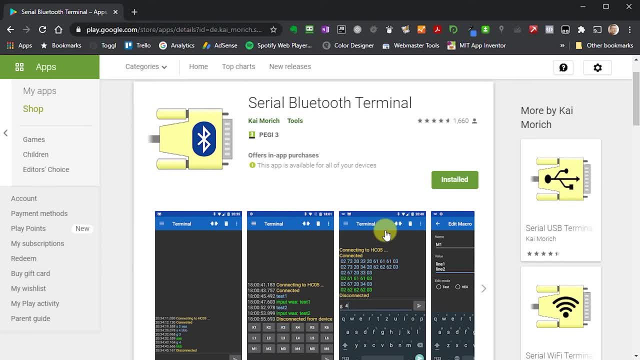 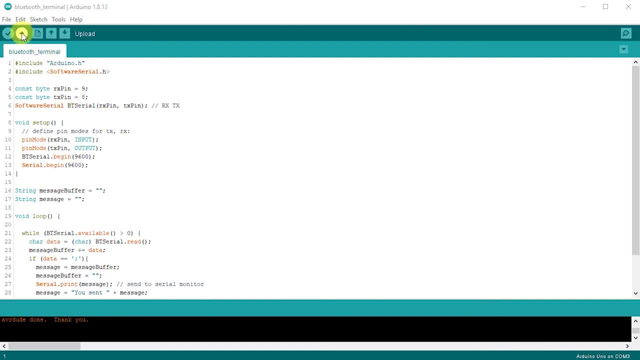 your phone and we'll be ready to start communicating with our Arduino. So if we come into our Arduino IDE, we of course need to upload the software up to the Arduino IDE. So we need to upload the software up to the Arduino IDE. So if we come into our Arduino IDE, we of course need to upload the. 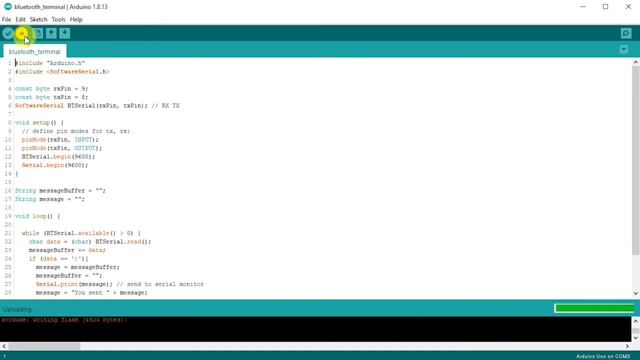 Arduino. So let's do that. And once that's up, we'll need to open up our serial monitor so we can actually see what's happening. So again, making sure we're on there and making sure we've got 9600 bauds selected, which is what we set our serial channel to work at. So now we should be. 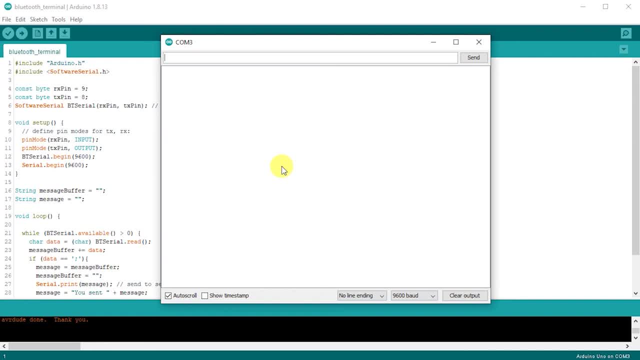 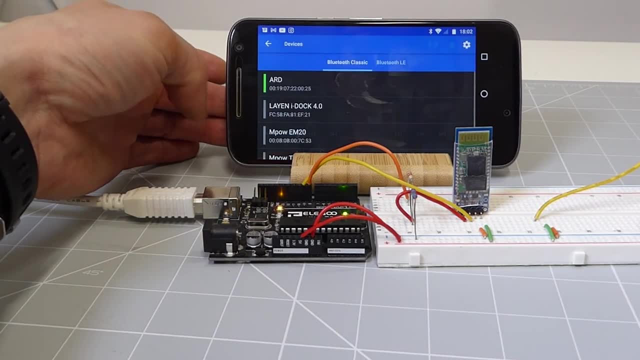 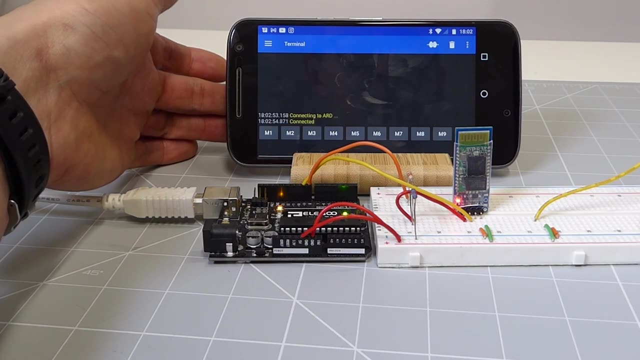 ready to actually make a connection with our device. So I've got the serial terminal up and you can see that it's sitting there waiting to connect to the Arduino. So if I select that, and now we've got a connection, So you can see that our red LED has stopped flashing. 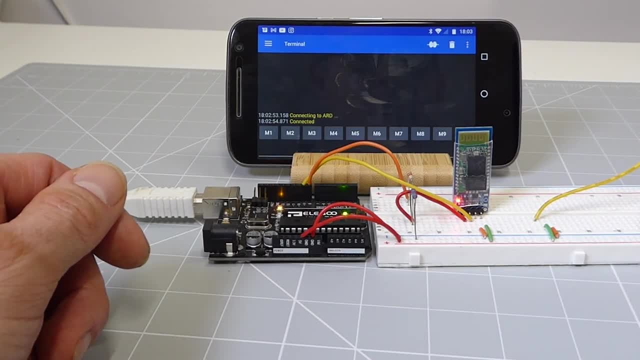 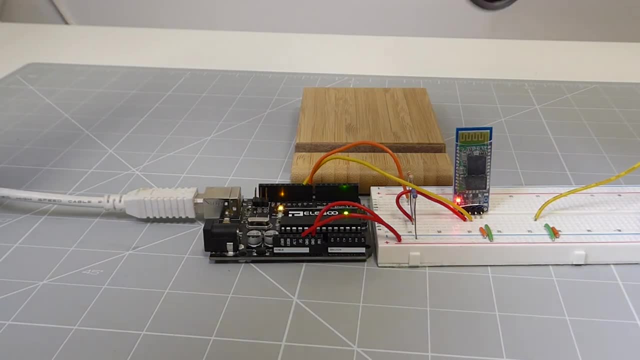 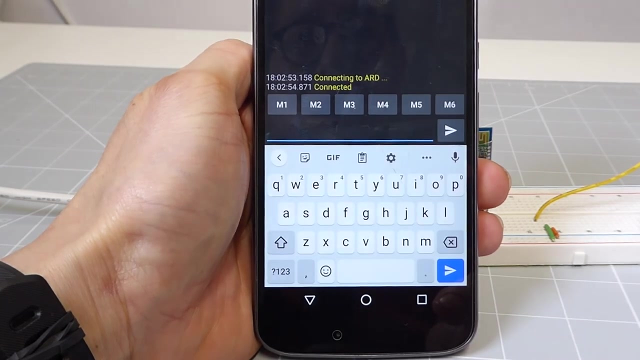 and is now on solid, And that means it's actually connected and ready to talk. So let's see if we can then do a message. Let me just grab hold of the phone a bit better and bring that forwards. Okay, So if I come in to here and start typing, 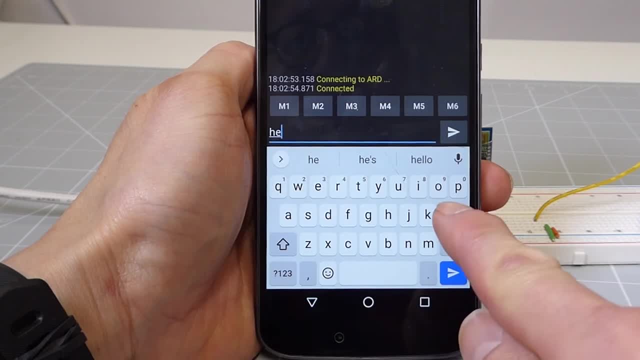 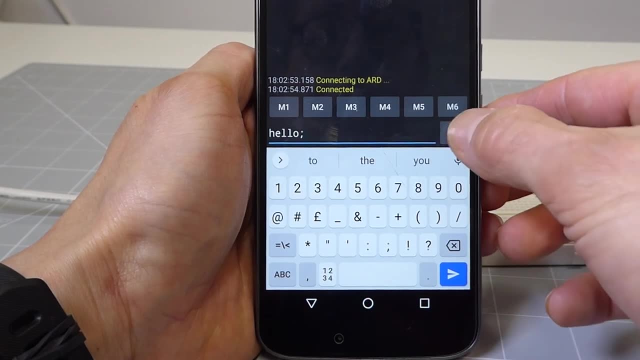 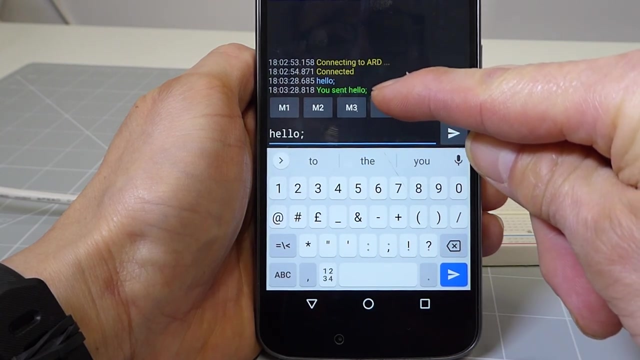 a message. So remember, we said that we were going to type a message and then we were going to use a semicolon to denote the end of a message. So if I send that, we can see that it sent hello. The Arduino has then replied with the you sent hello. And if we go back into our serial terminal, 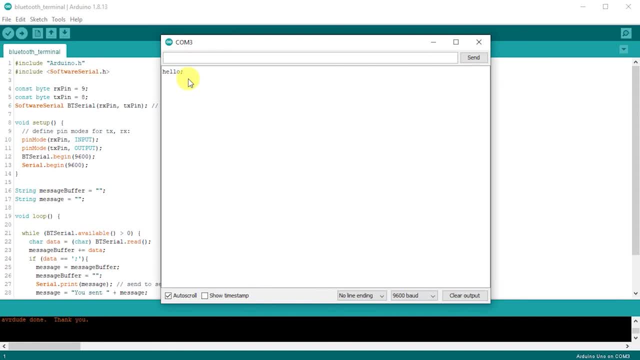 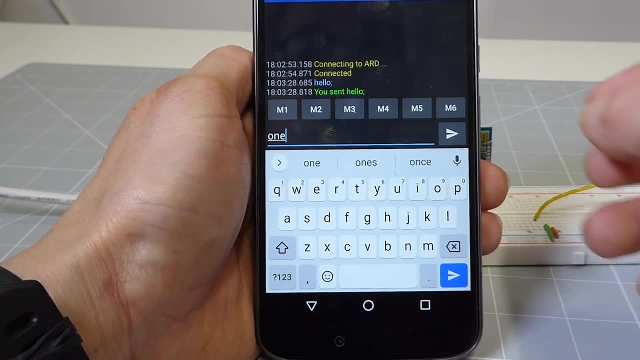 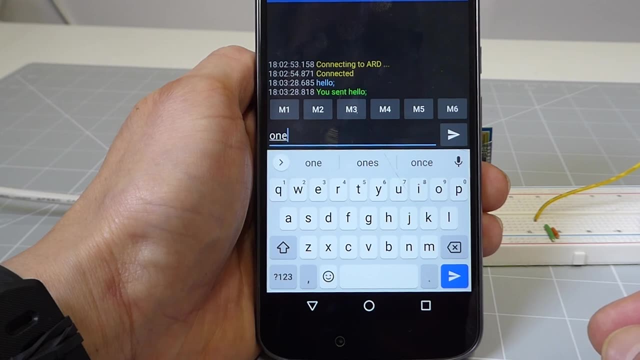 we can see that we've got the message coming up here, So we can then, if we come back, we can then send a number of messages. So if we send one, if we don't put a semicolon in, remember our code was simply going to collect any characters you send and then build them up. 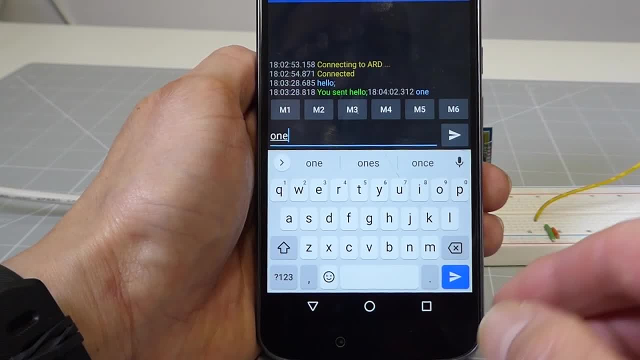 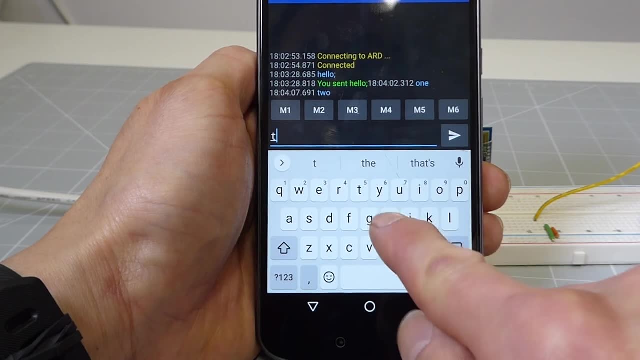 into a message. So I could actually send a number of lines first, like this: So you can see that we have sent in one, two and then three, And at this point I'm going to send the end of message character and send that in. 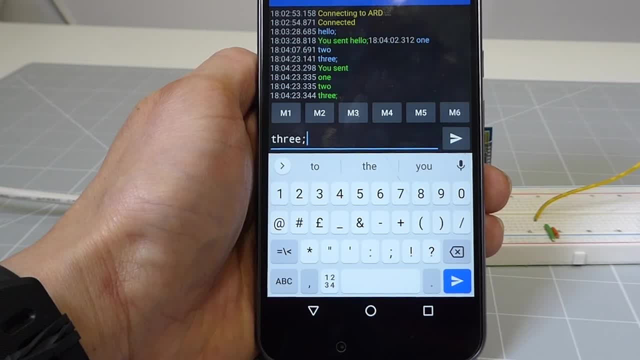 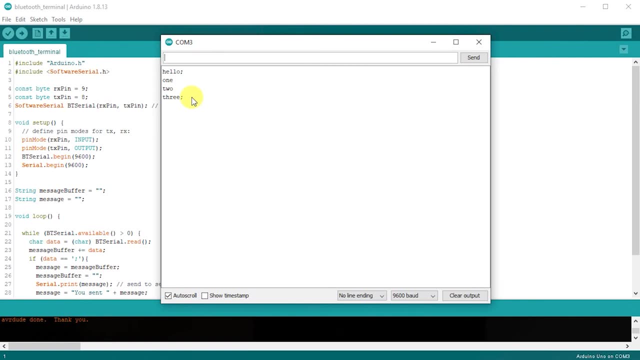 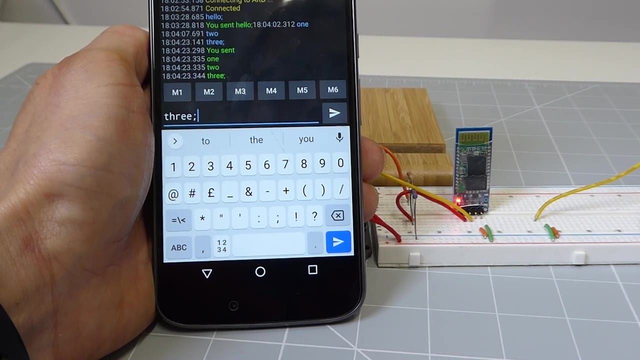 And you can see that it's now come back saying: you sent one, two, three And on our serial monitor you can see we've got those three lines that were all buffered up waiting to be sent. So we've got our Bluetooth module. It's now connected up to our Arduino. It's now paired. 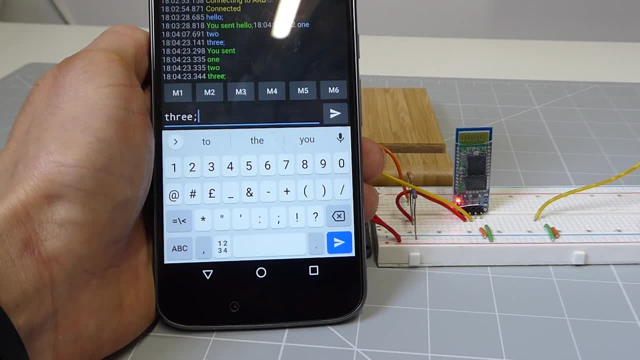 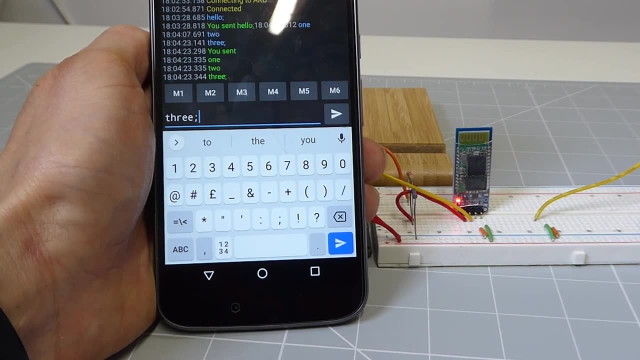 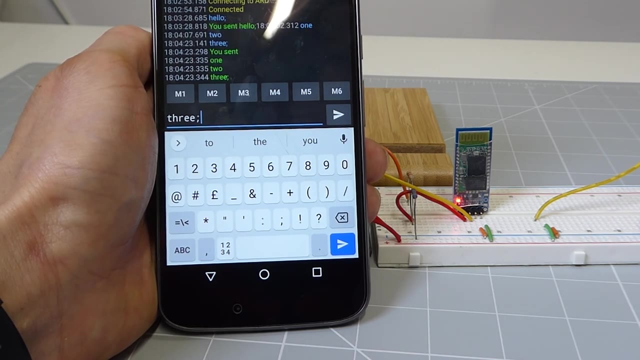 with our phone. We're now able to both send information from the phone down to the Bluetooth module and then into the Arduino, And we're able to send information up from the Arduino through the Bluetooth module into our phone, And that is the basic setup for any of your Bluetooth communications. 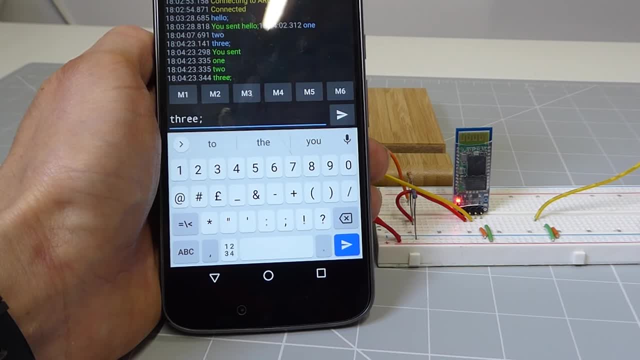 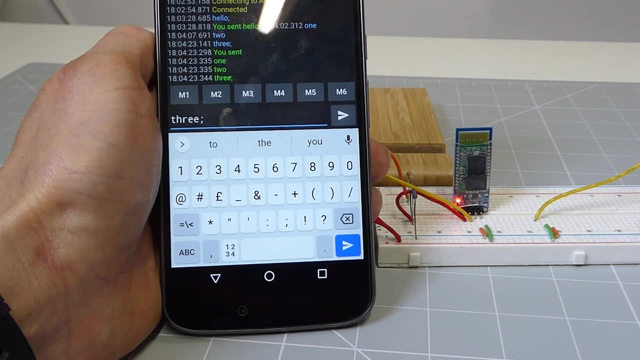 All we're simply going to be doing is using the Bluetooth to simply provide a serial channel between our Arduino and an app running on your phone or your computeror any other Bluetooth device. The communication we're going to send between the two will all be. 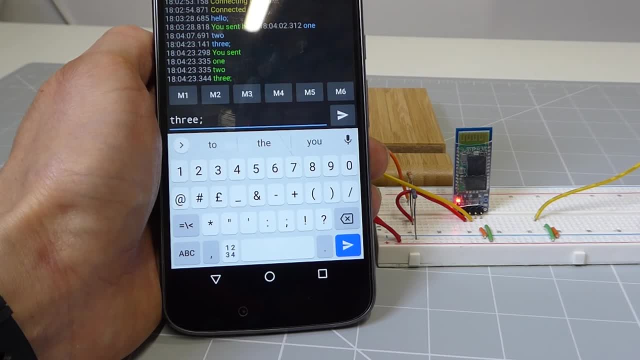 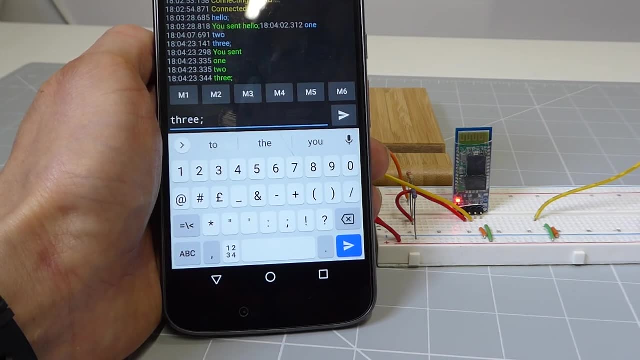 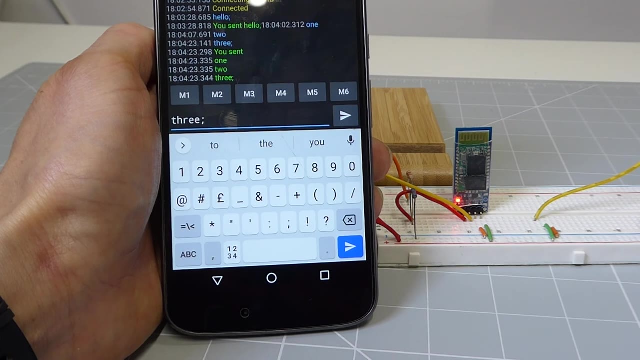 in terms of character information or individual bytes. So we can send numbers up or we can send strings of characters, And again, it's then up to us to interpret what those messages are and how to both encode them, to send them between devices and decode them once they arrive. And that's really. 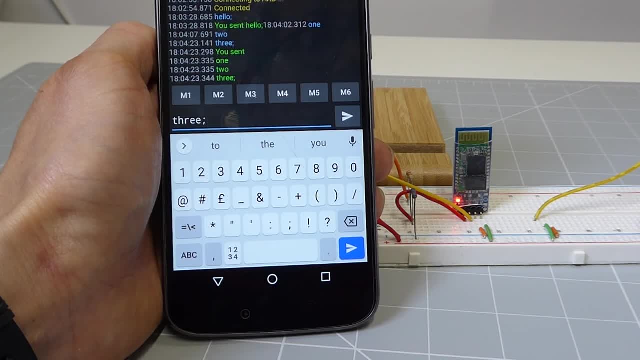 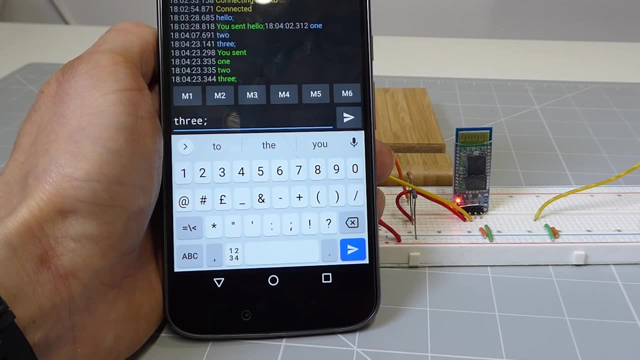 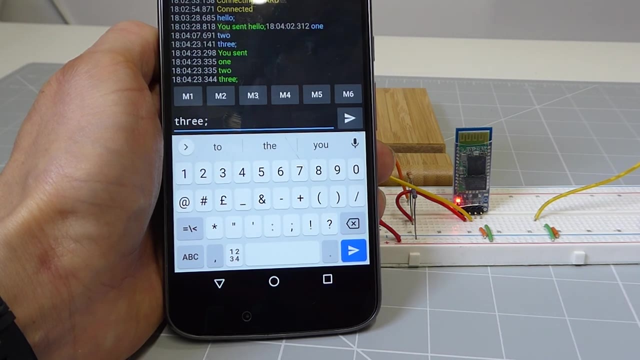 what we're going to look at in the very next lesson. So we're going to use this as the basis then, And we're going to expand that up. I'm going to show you how to very quickly put together an app running on your phone using a very useful piece of software from MIT which lets you very 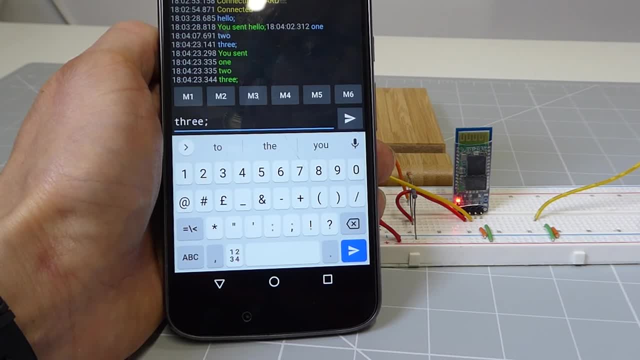 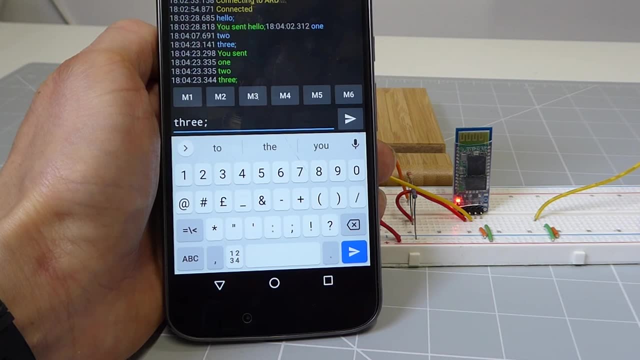 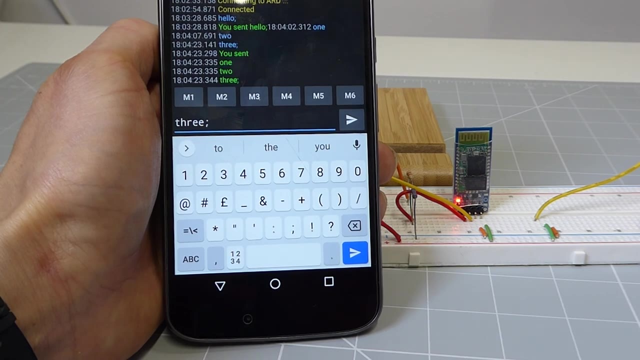 quickly build those And we're going to then control some RGB LEDs and we'll see how we can use some sliders and user interfaces on our phone to do that. But make sure that you're have a look at the course pages on my website Again, links in the description below And there. 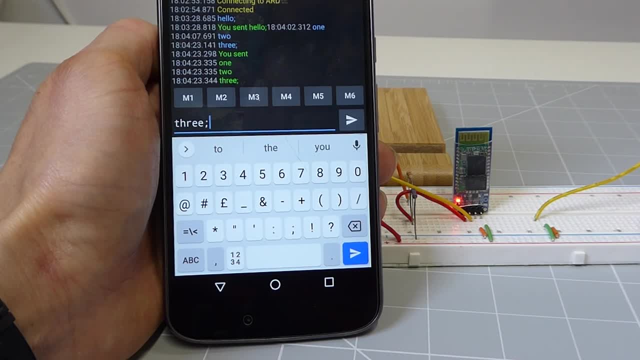 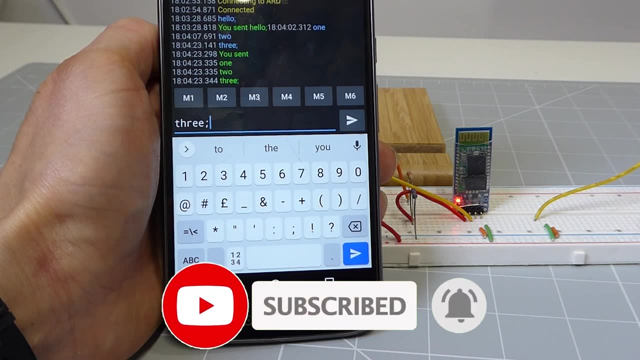 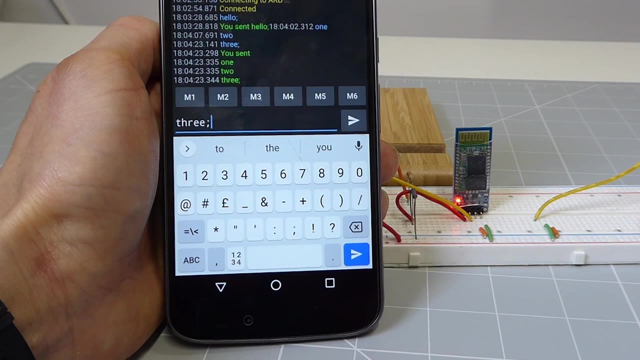 you can download any software we've done here and again, get circuit diagrams and so on. If you've enjoyed this, do please leave a like and subscribe to the channel. Every subscription helps build what I'm doing here And then hopefully I will see you in the very next lesson. Bye for now. 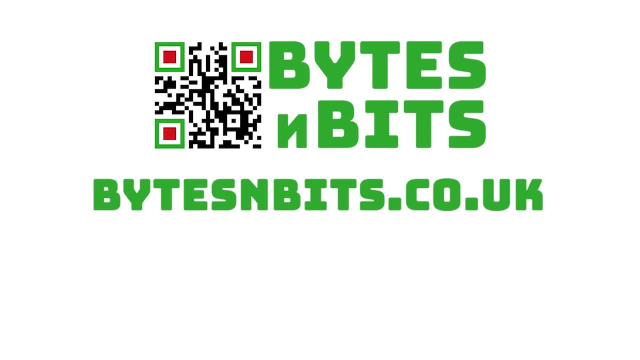 Don't forget to visit the course pages for this project. There you'll be able to download the code for this lesson and get lots of extra hints and tips. You'll also get access to all my other programming, electronics and gaming projects. All the links are in the 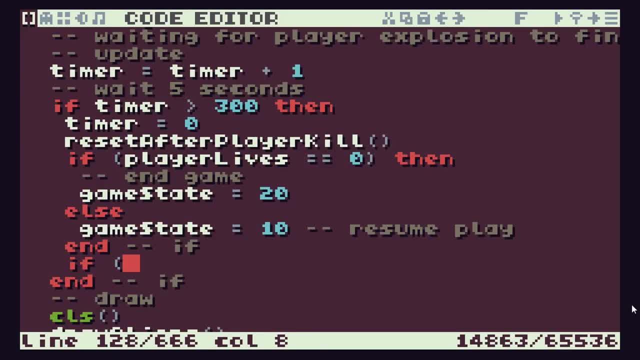 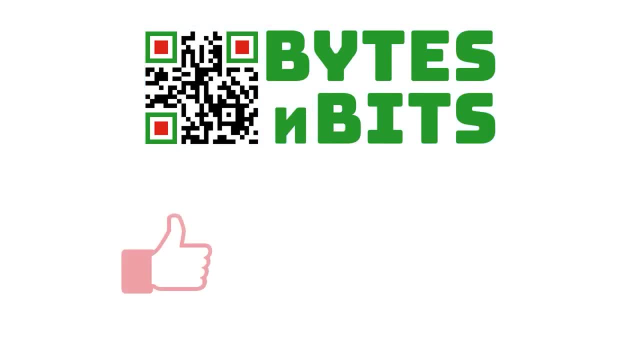 description below For more games, programming, electronics projects and retro gaming. please make sure you like this video, subscribe to my YouTube channel and visit my website And I'll see you in the next video.